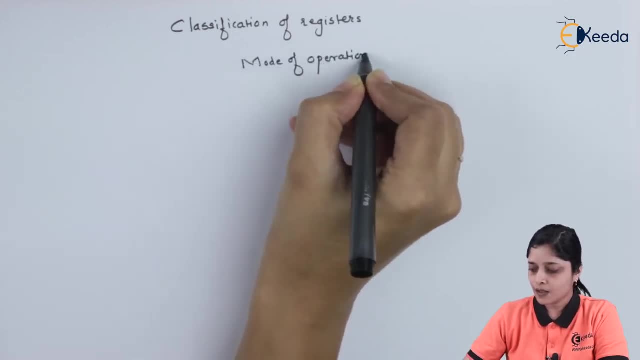 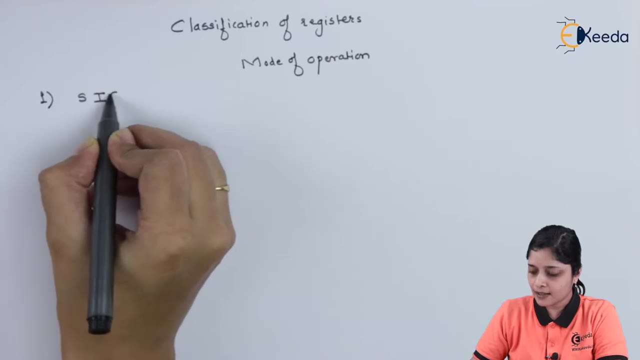 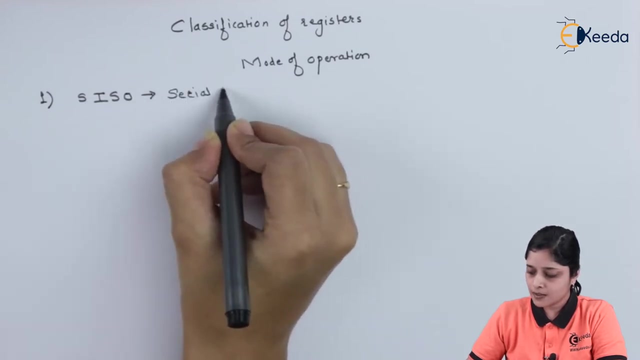 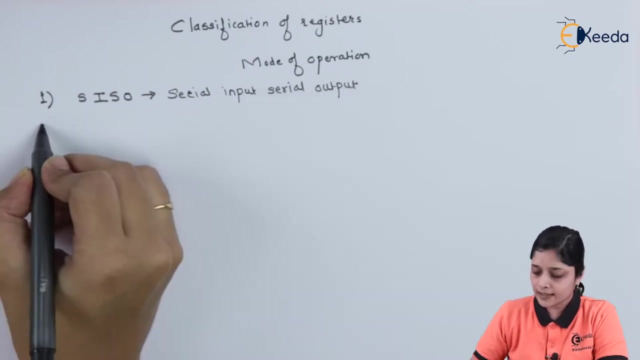 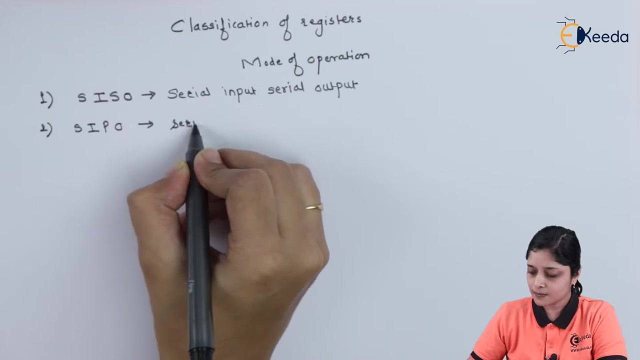 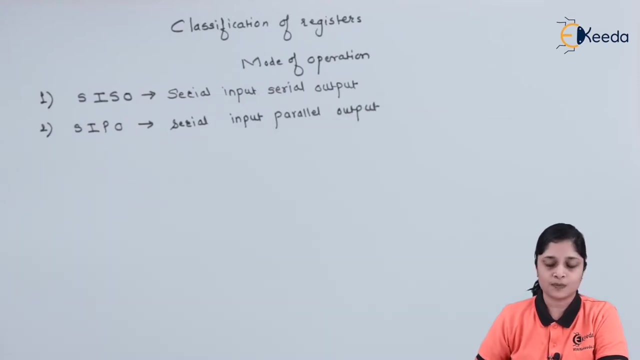 the mode of operations. So first case we will discuss here is what SISO? What is the meaning of SISO, Serial input, Parallel output? Next is SIPO. It is called as serial input, parallel output. The third one is PISO, The long form is parallel input. 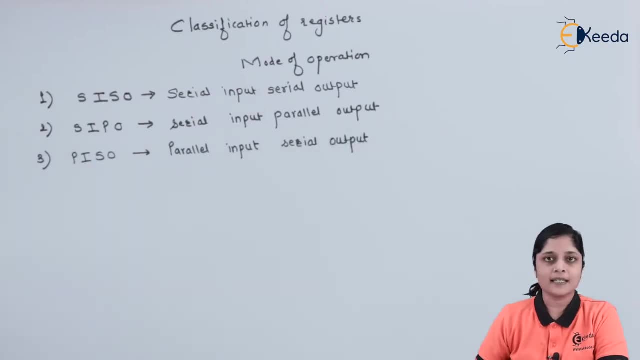 Serial output. And last one is PIPO, That is, parallel input, parallel output. Now, with the help of all these three cases, we can give the input to the system bit by bit, So that is either serially or parallely, And at the output according to the applications. 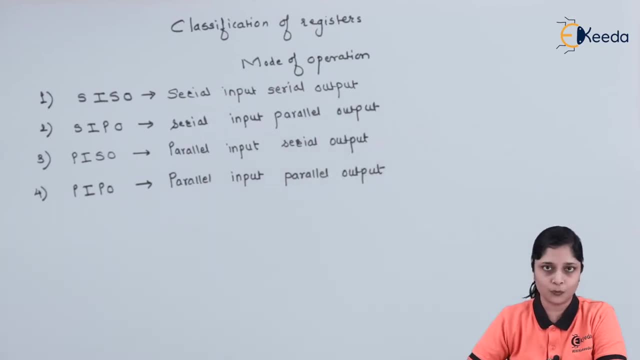 you can get the output by serial output or the parallel output And according to these two formats, we have four types of classification of resistors, That is SISO, SIPO, PISO and PIPO. Now we will discuss the first one, that is SISO- Serial input, serial output. So 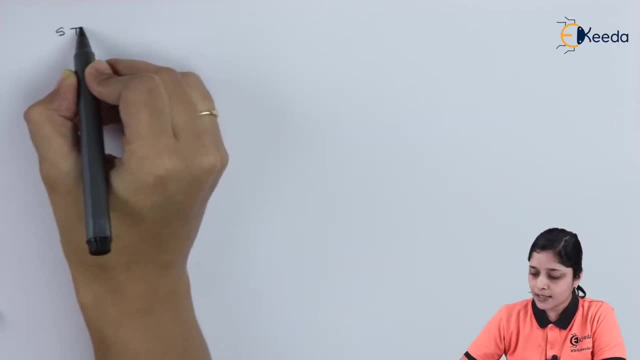 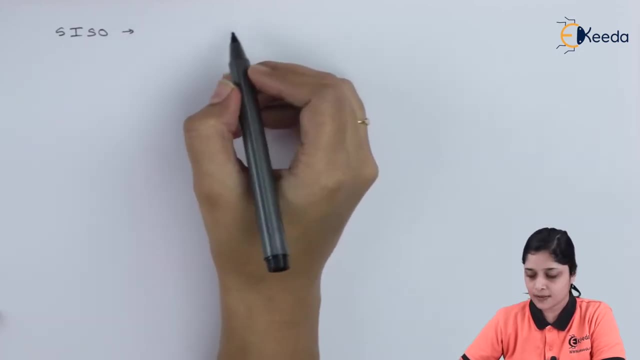 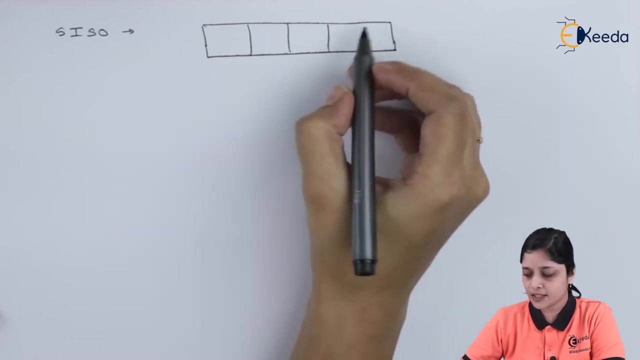 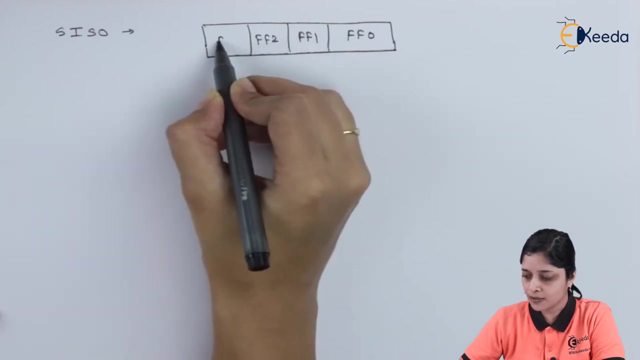 for SISO serial input, serial output. flip flops are used for this process. Suppose you have four number of flip flops connected one after another. This is flip flop 0, flip flop 1, flip flop 2 and flip flop 3.. So here flip flop becomes the basic building block for the 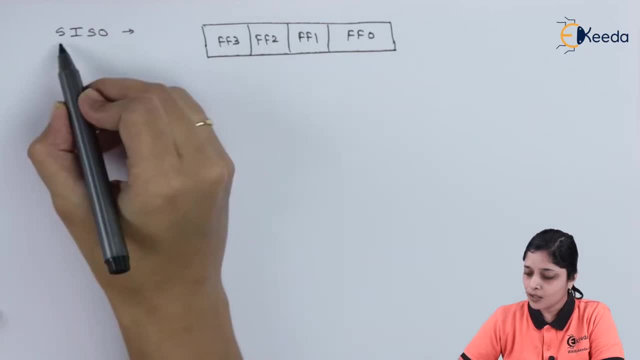 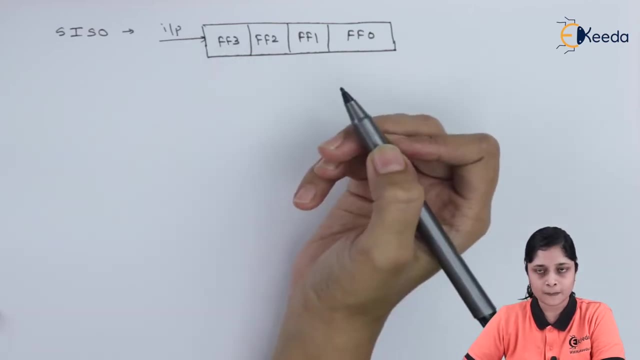 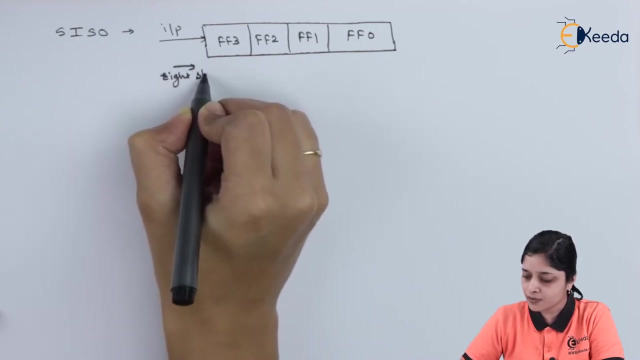 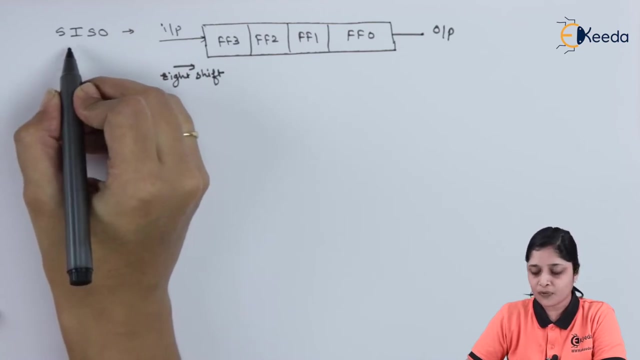 designing of resistors. Now, serially you have to give the input. So here we can give input to flip flop 3.. If we want to move towards right, then it is called as right shift And here you will get your output. So this is the type of SISO right shift: One by one you 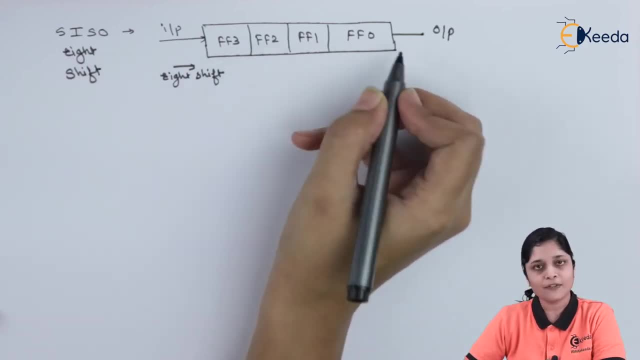 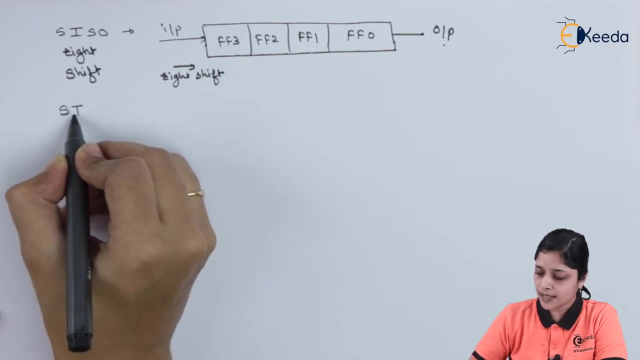 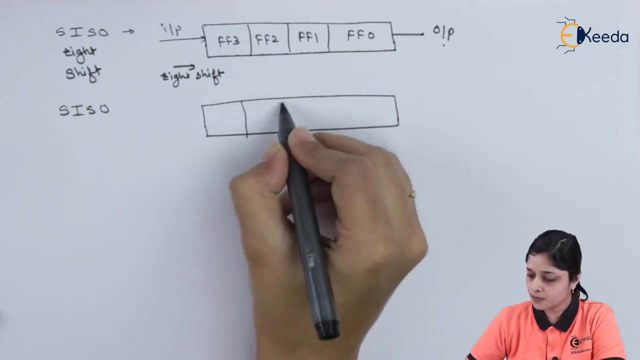 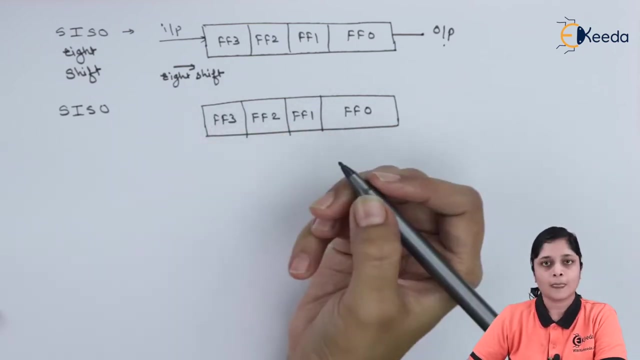 one bit is going inside the each flip-flop and finally you can get your output. at this stage now, SISO, that is, serial input, serial output. this is your flip-flop zero. now we have done with the right shift. now we will focus on what left shift. 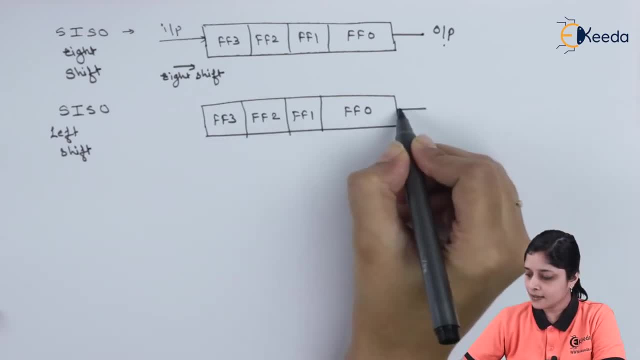 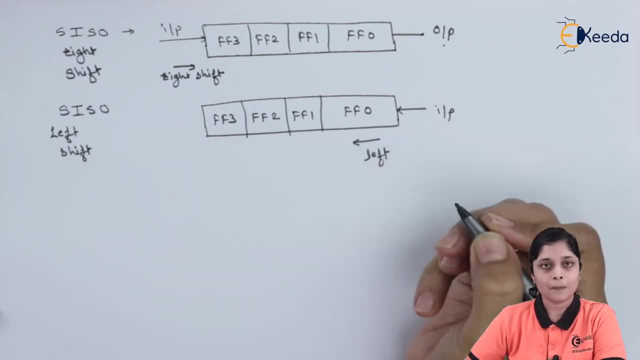 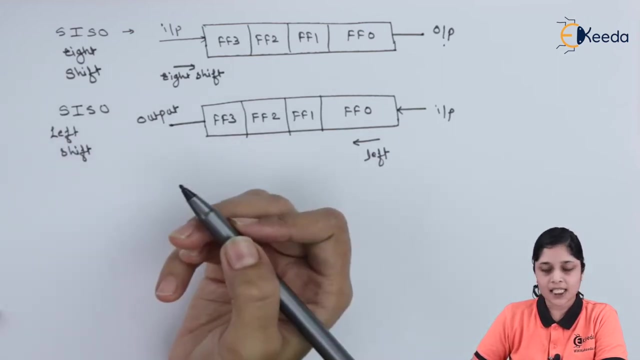 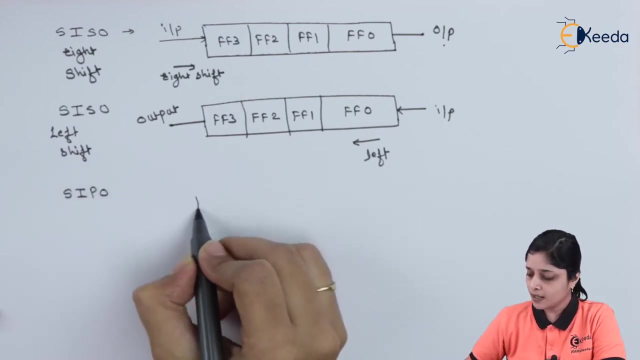 means here you have to give the input and data will be moved towards the left side, bit by bit, and here desired output you will get. in this way the binary bits are processed. now we have done with SISO, now we have SIPO again. we have resistor consisting of four number of flip-flops. 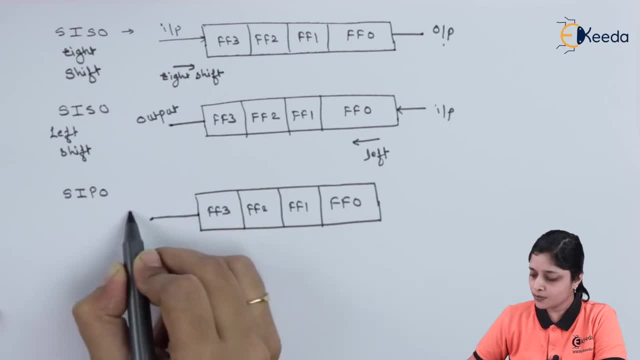 so serially you have to give the input. so input you have to give at this stage and parallel output you want. so from each flip-flop you want output. this is done by getting them in parallel way. so this is your output side. in this way you can get your data parallelly. so we have achieved serial. 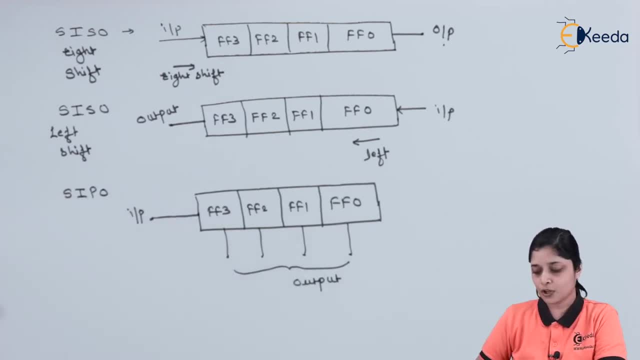 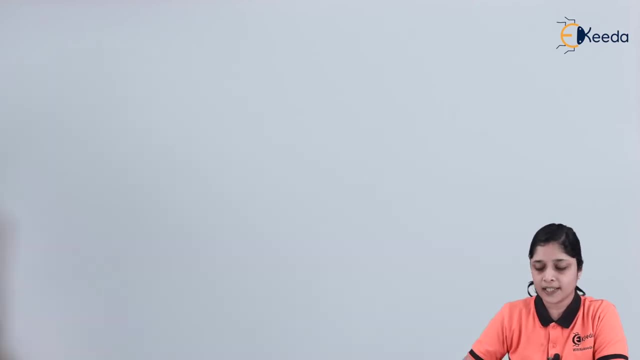 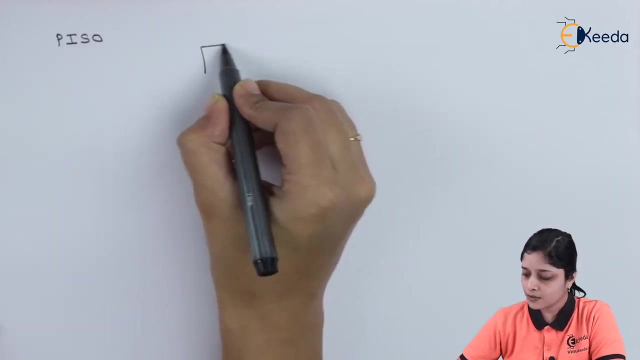 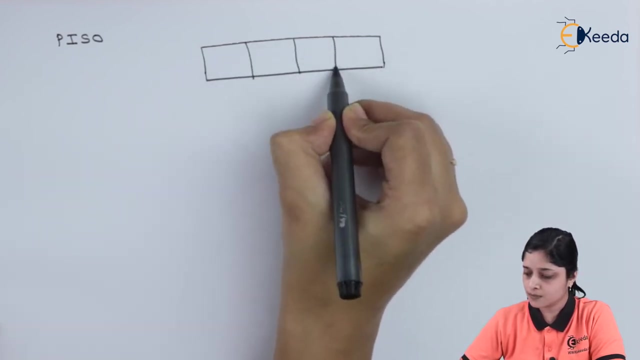 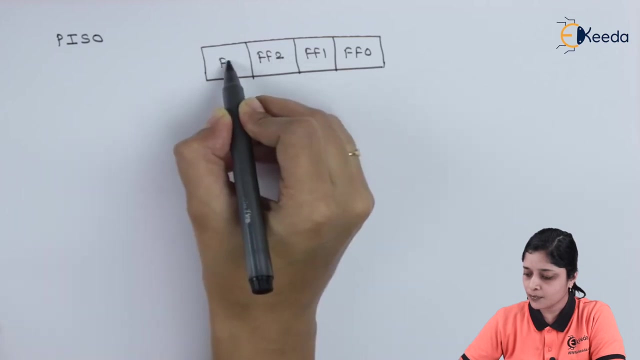 input, parallel output. now. the next is what parallel input, serial output. now let's discuss. so we will right here. parallel input, serial output. again in. you have to take a register consisting of four number of flip-flops. this is flip flop 0. this is flip flop 1, flip flop 2 and flip flop 3. here the input side you. 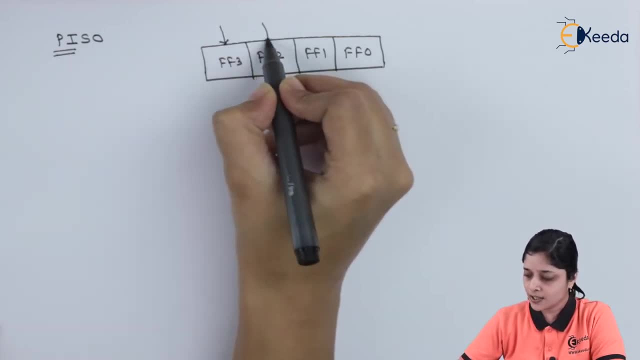 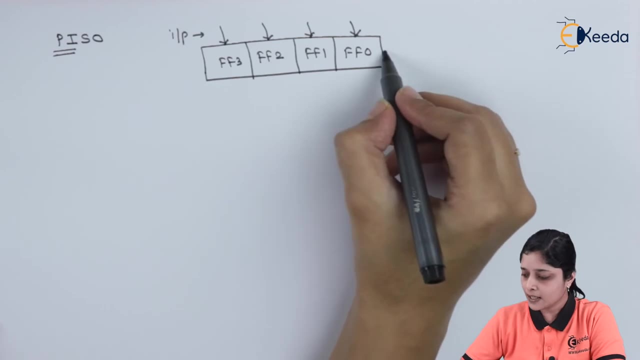 have to give parallelly. so in this way you can give the inputs parallelly to each flip-flop and output you have to take serially. so in this way serial output you can take by connecting the output to the last flip-flop in this way. 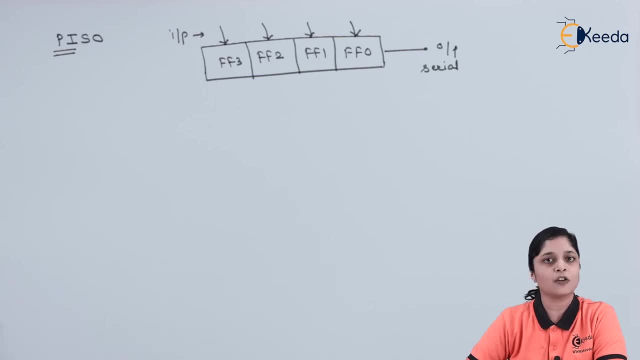 you can achieve input parallelly and getting output serially. now the next type is what? parallel input and parallel output? if, according to the application of the input side, you have to give a serial output to each flip-flop applications, the requirement is of what? getting the output parallelly and giving 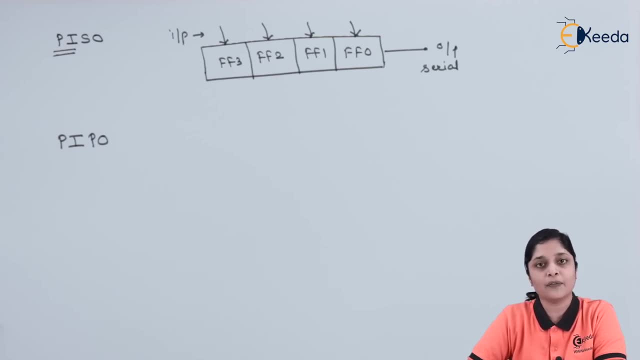 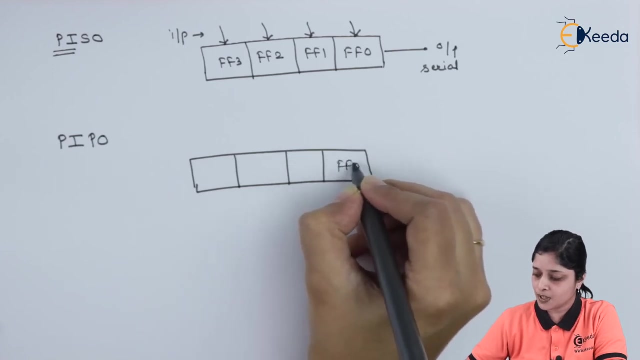 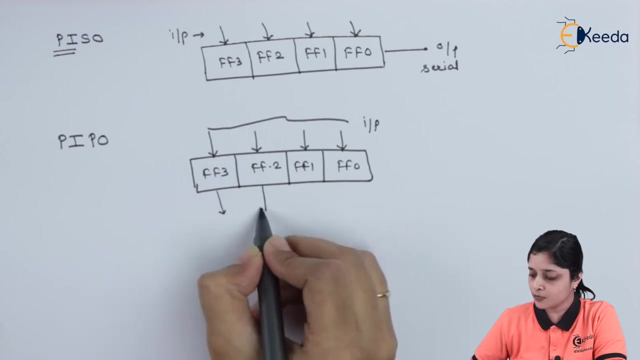 input also parallelly, then in what case you have to design again? you have to take four number of flip-flops, that is register. this is flip flop 0, 1, this is 2 and this is 3. ok, so this أو input or output water that you have to give is the. 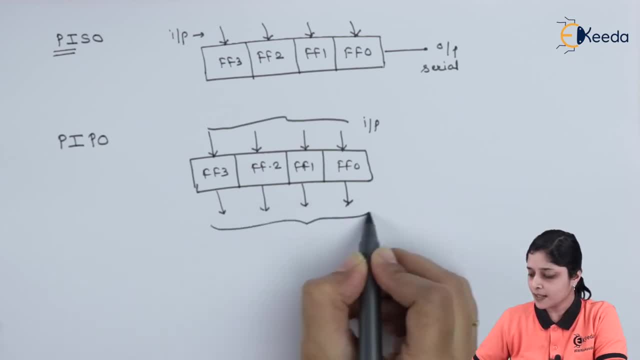 t help letter, which I in the root right, so in in time field is equal to 0 and input is equal to enter at base P M. sorry, input and output at base P M. this is the approaches name. if you own scribe, this is Scrapbook present. these arešl approaches. by this will give out some direction in not to Tenor Press liter. so these are word. So all these are the classifications of resistor based on the mode of operations. It also depends upon the applications you want to use, and hence there are four types: serial input, serial output. serial input- parallel output- parallel input- serial output. 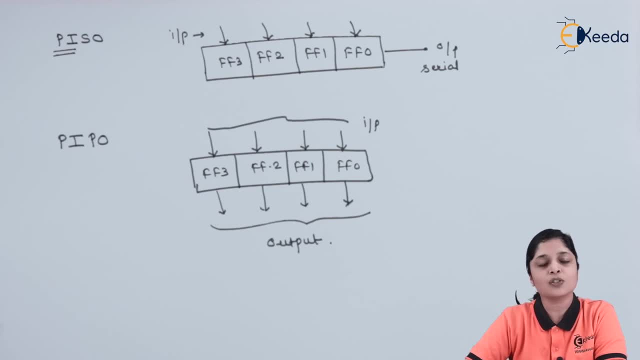 and parallel input, parallel output. This is all about the classification of the resistors. Thank you for watching this video. Stay tuned with eKIDA and subscribe to eKIDA.